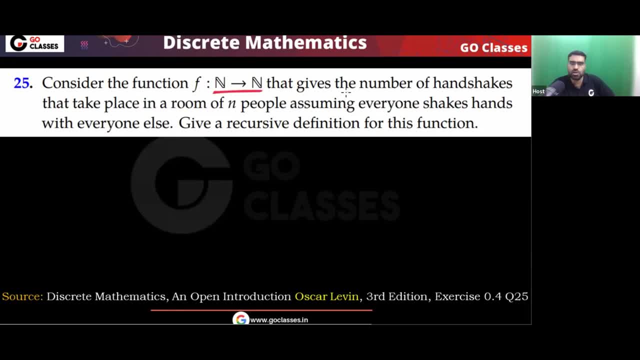 Consider the function from n to n, From natural numbers to natural numbers. Consider the function that gives the number of hand sex that take place in a room of n people, Assuming everyone sex hands with everyone else. So this is the point. This function is basically telling you how many hand sex are there in a room of n people if everyone sex hands with everyone else. Give a recursive definition of this function. 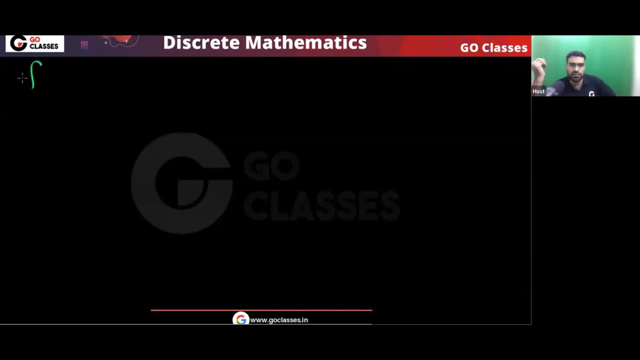 First you understand this function. First you understand this function. This function is from n to n. This is your n, this is your n. Now we are saying that what this function is telling you. please tell me. Like, for example, if you take a value like, if you take a value 5, then what f5 will tell you? What this f5 will tell you Tell me, It will tell you how many hand sex are there if five people sex hands with each other. Please read this question. 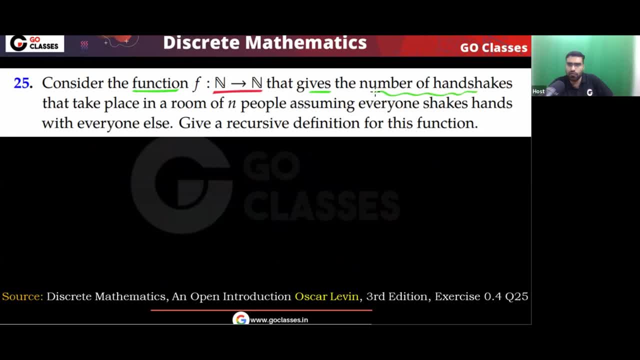 This function gives the number of hand sex. This function gives. this function gives. this function outputs- Please read this: This function outputs the number of hand sex that take place in a room of n people, in a room of five people, in a room of five people, Assuming everyone sex hands with everyone else. So please understand, this function gives. the output of this function will be: the output of this function will be number of hand sex. 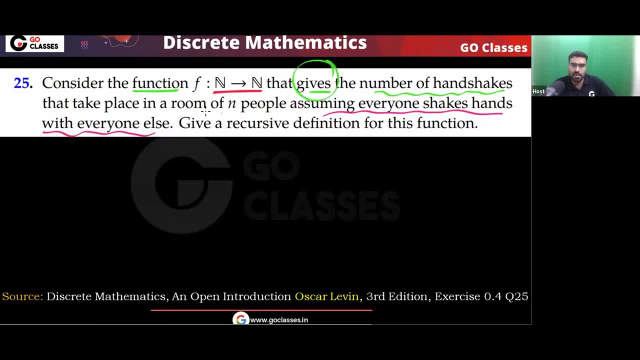 For this function, the output will be number of handshakes in a room of n people. I am taking n equal to 5.. So in a room of 5 people, assuming every person shakes hands with everyone else. So you tell me what f5 will tell you. 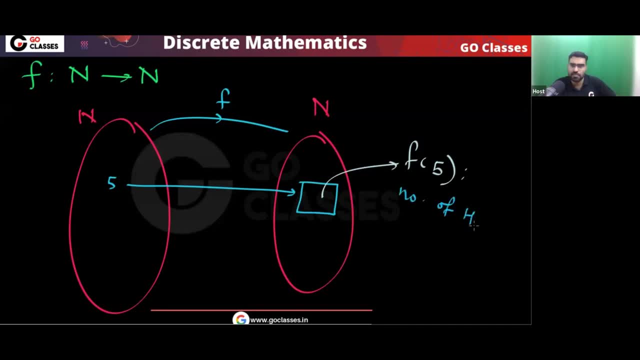 This f5 is basically the number of handshakes. the number of handshakes in a room of, in a room of 5 people where everyone shakes hands with everyone else, where every two people shake hands, where every two people are shaking hands, where every two people. 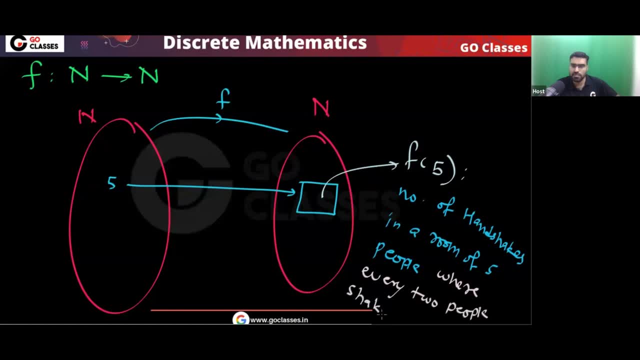 shaking hands. shake hands, So this is f5.. Is this point clear? So this will be the f5.. Means f5, the output: This function will give you f5.. This function will give you number of handshakes. 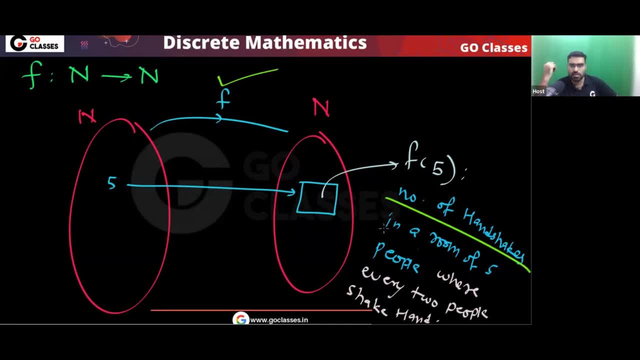 This function is going to give you number of handshakes in a room, in a room in which you have five people. So tell me, in a room, if you have only one person, how many handshakes are possible If you have only one person, if you have only one person in a room, if you have only one. 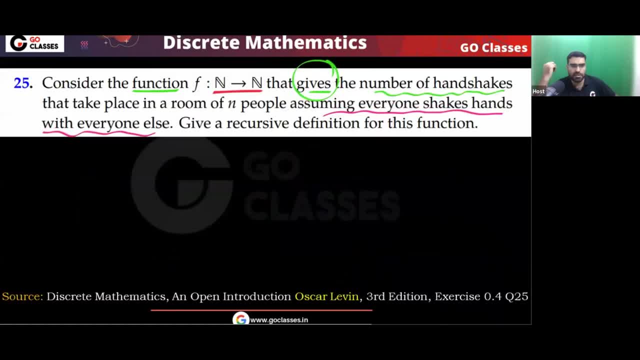 person, then zero handshake is possible. Remember here: handshake with everyone else You cannot handshake with with yourself. Okay, You cannot, You cannot handshake with yourself. The question is saying: everyone else You cannot handshake with yourself. Don't do that. 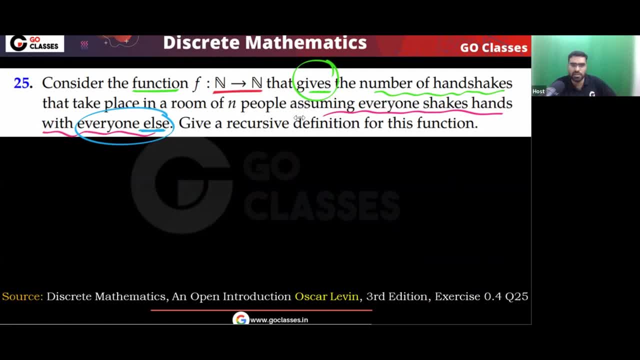 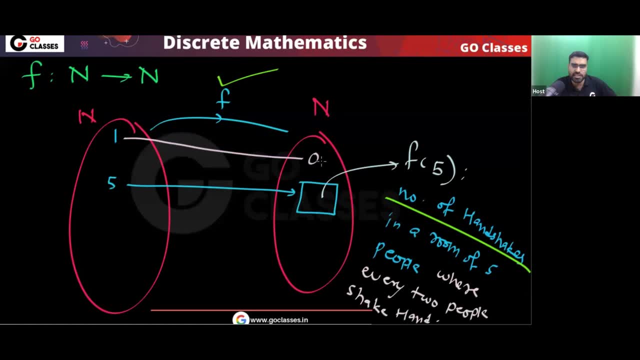 That is weird. People will think that you are maybe mad or something. You are crazy. So anyway, so you can see with everyone else. Now you tell me so if you have only one person, how many handshakes will be there? 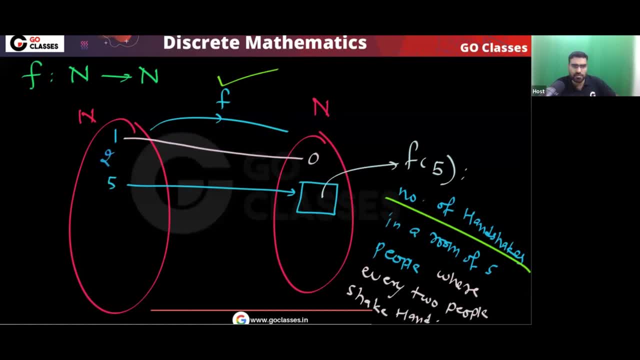 There will be zero If you have two people. how many handshakes will be there If you have two people? if you have two people, only one handshake will be there. If you have two people, only one handshake will be there. 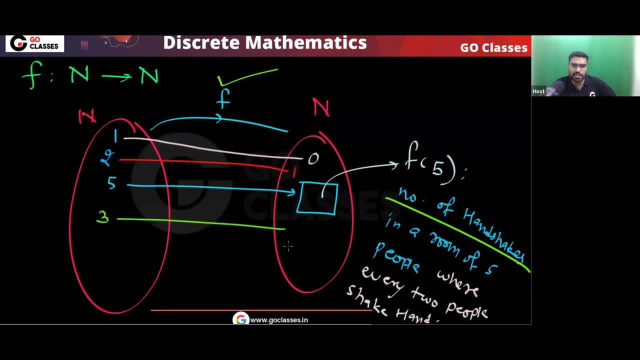 If you have two people, only one handshake will be there. If you have three people, how many handshake will be there? If you have three people, there will be three handshakes. If you have four people, think about it: How many handshake will be there? 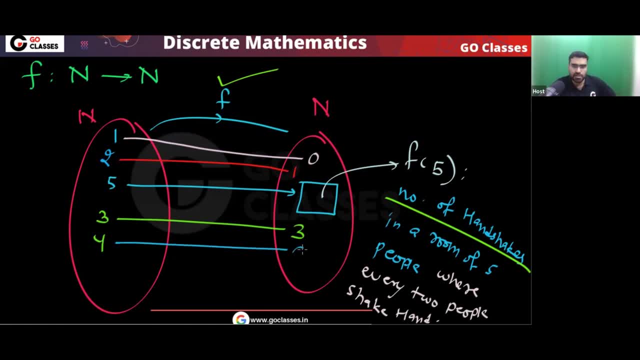 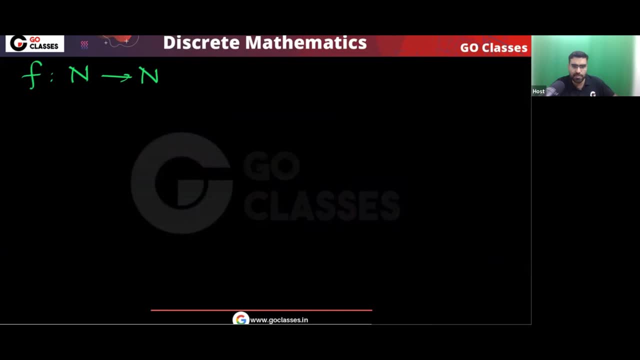 Think about it, I will tell you the answer. But think about it, There will be total six handshakes. Okay, Anyway, we will see what is happening here. See, very easy things is happening. You tell me simple point, very simple point. 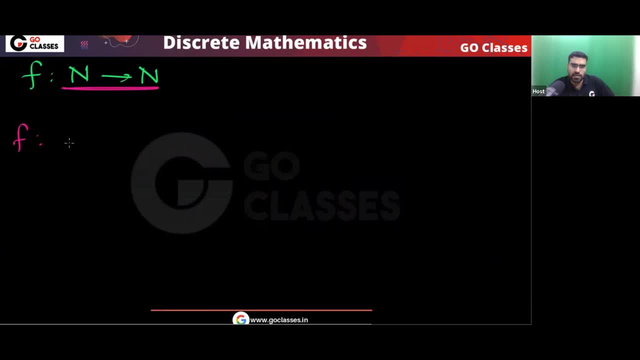 You tell me this function we have Here. I am saying number of people like one, two, three, four, five, six, seven, eight, nine. one, two, three, four, five and N plus one and so on. Okay, So you tell me and this: 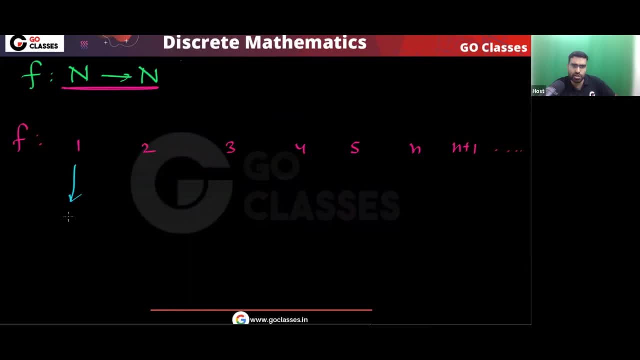 is your function. So if you have one person, number of handshake will be zero, right? If you have one person, then number of handshake will be zero. If you have two people, then number of handshake will be one. If you have three people, number of handshake will be. 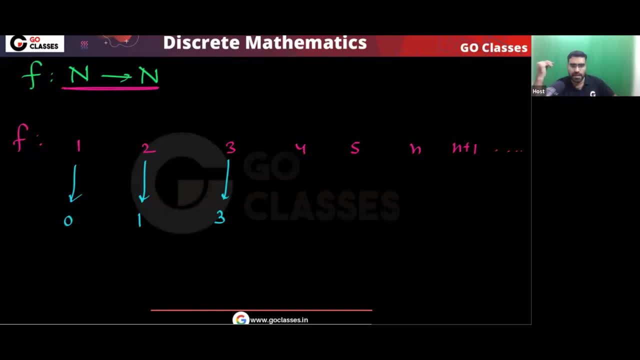 three. Now you notice Now one thing: you tell me if there are in this room already there are, let's assume, N people, I don't know how many handshakes will be there, I don't know, I don't care, I do not care. Let's assume in this room there are N people and 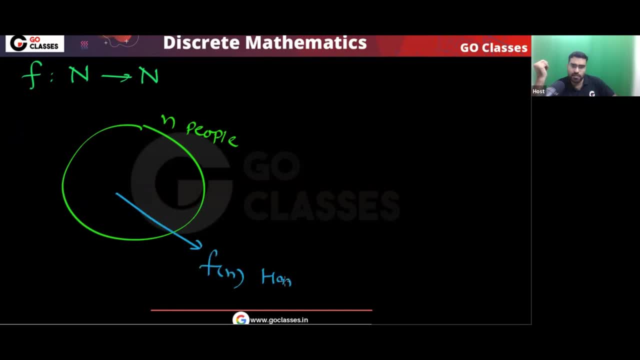 let's assume there are FN handshakes. Let's assume I don't know what is this FN. I don't know, I do not, I do not know what is FN. So you tell me there are total N people in. 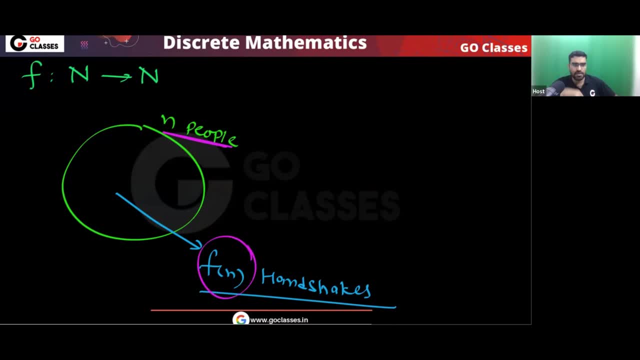 this room. Let's assume there are FN handshakes. Now one more person comes. Now one more person comes in this room. Now one more person comes in this room means: now you have total n plus one people. Now you have total n plus one people. 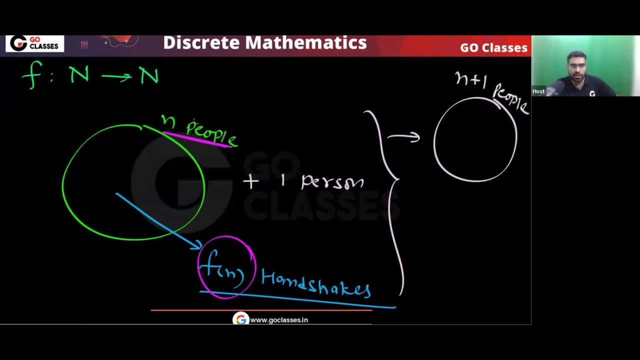 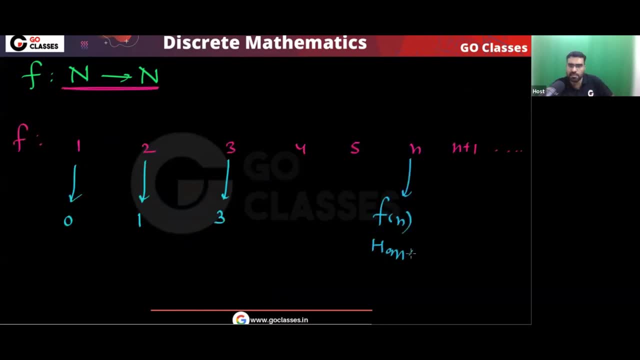 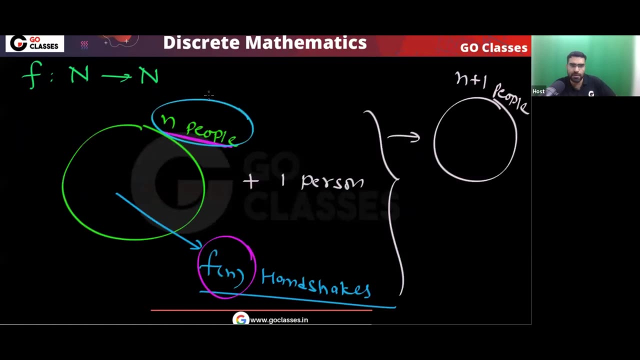 Are you getting my point? See, when there are n people, let's assume fn handshakes are there. When there are n people, let's assume there are total fn handshakes. total fn handshakes are there. When you have n people in a room, in this room, there are n people, this is your room. 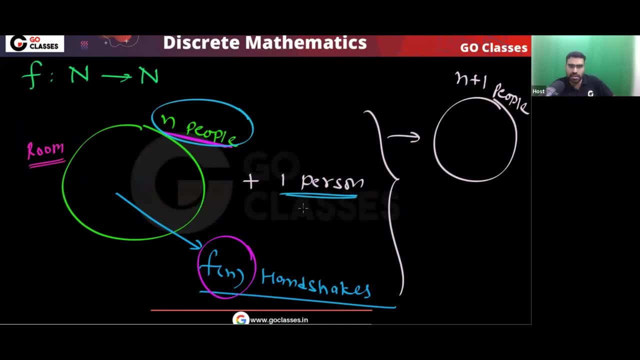 okay, Now, if one more person comes, one more person enters, one more person enters, then you tell me: already, there are already, already already these people. these people did they handshake with each other. These people did they handshake with each other. yes, 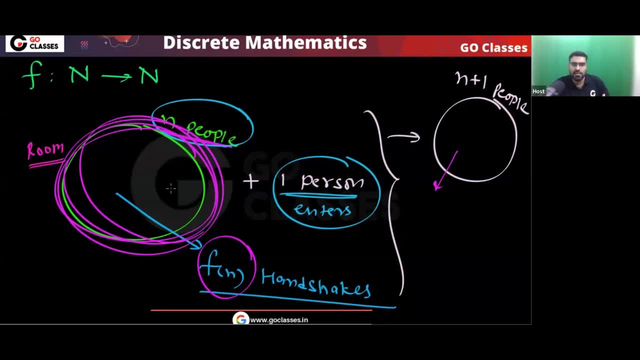 So will they? will they handshake again These people? they are handshaking with each other. no, So already before this, before this, This new person came, This new person, before this new person came, already fn handshakes were there. 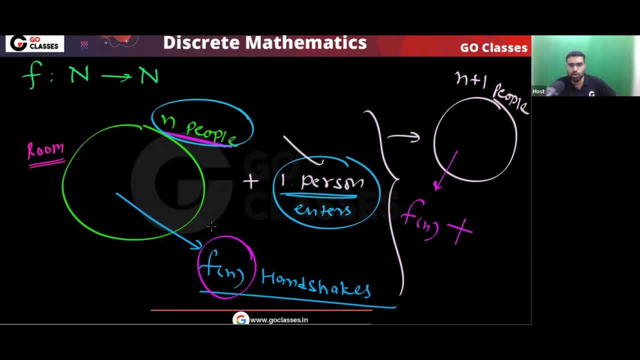 Because of this one new person. how many more will be there Because of this one new person. this new person will handshake with all of them. This new person, he will handshake with all of them. He will handshake with all the n people he will handshake. this new person will handshake. 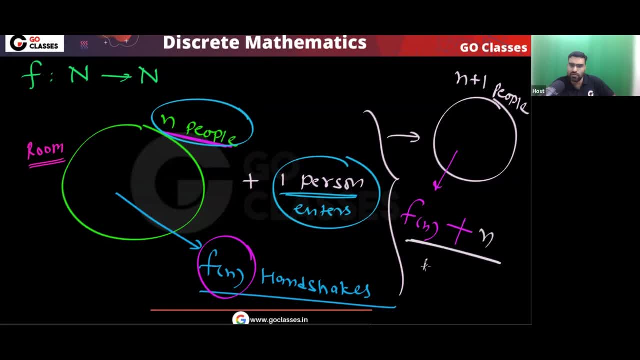 with all the n people. So these many handshakes will be there. Right Simple, isn't it simple that these many handshakes will be there, very simple. So this new person will handshake with all the remaining people, So there will be total new, I can say, and new handshakes will be there. 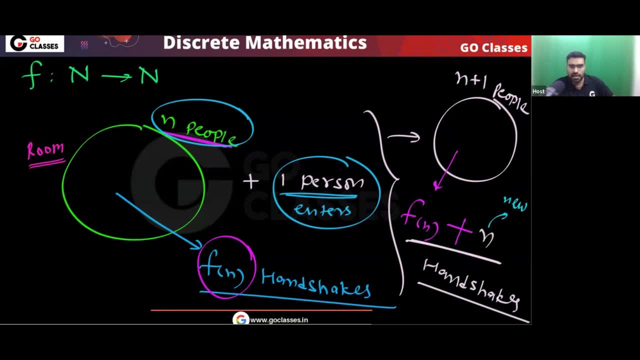 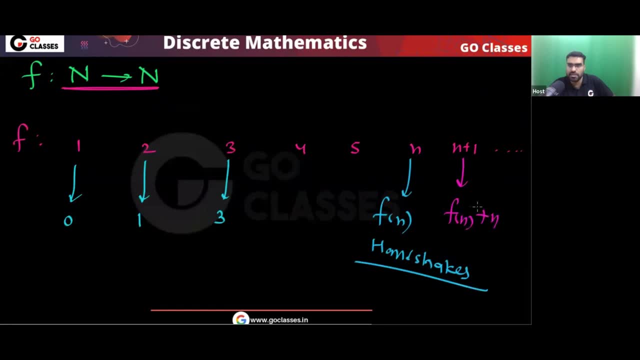 These are the new handshakes. So finally you are getting. I can say, when you have n plus one people, when you have n plus one people, then basically you are getting fn plus n, these many handshakes. Okay, so this is the recursively we got. 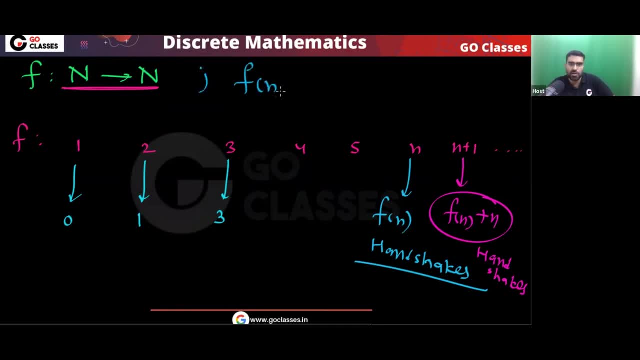 So we got this, we got this, that fn plus one, fn plus one, that is previous plus n. Okay, please understand. f of next, f of next, that is f of current plus n. f of next, f of next: this is the next f of next, that is, f of current plus n. 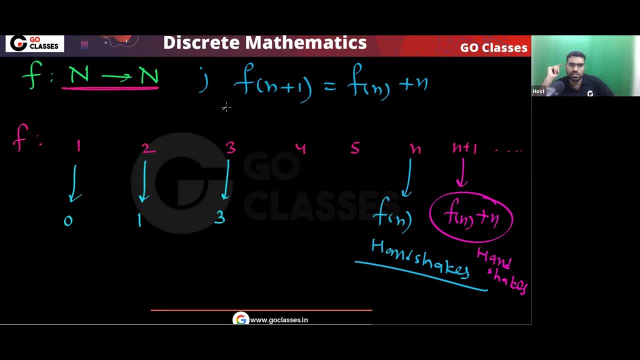 Okay, So, for example, when you are here, so for example, when you are here, then what is the next? f of next will be f of current plus n, So that will be six. or you can understand like this that f of current that is f of. 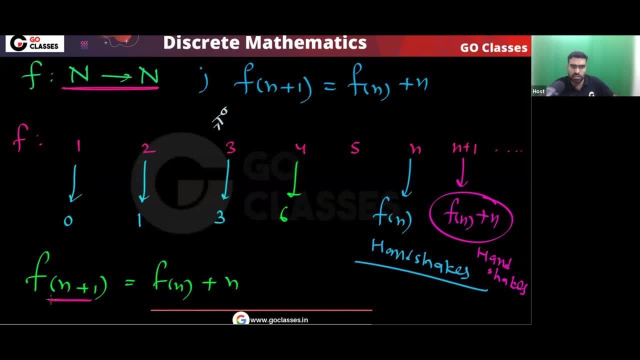 previous plus n. So if you think that this is the current, if you think this is the current f of current, that will be f of current, F of previous plus n. So, for example, what will be a five, If you are here, it will be f of previous plus n. 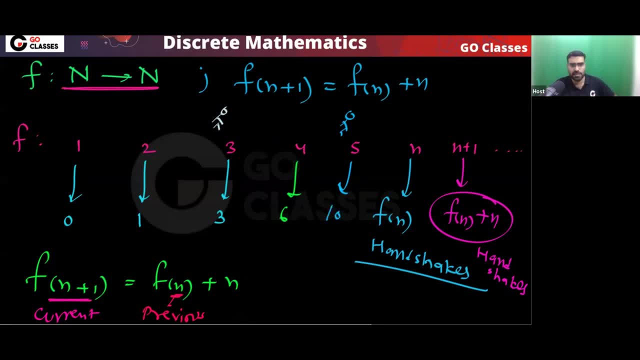 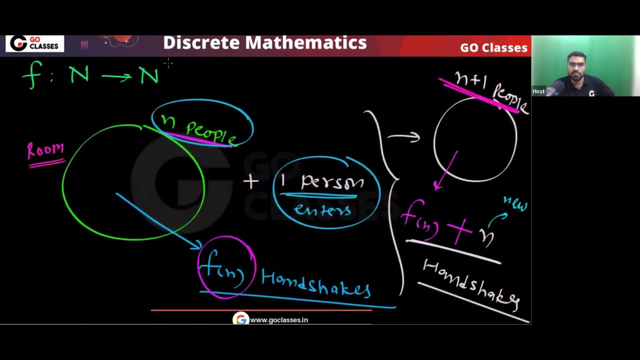 So that will be 10.. So, like this understood, This is a good question. but very simple question, but very interesting. This type of questions. of course this type of questions will come in the get exam. Of course this type of beautiful questions will come in the get exam. 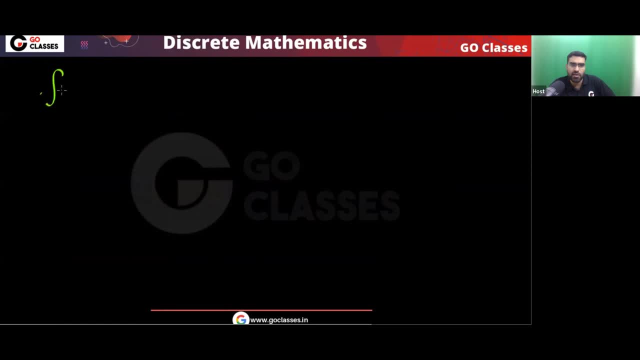 So, ultimately, what you got Ultimately, Now you can find what will be number of handshakes when you have 10 people. Now you can find, for example, f 10, you can easily find what will be f 10.. 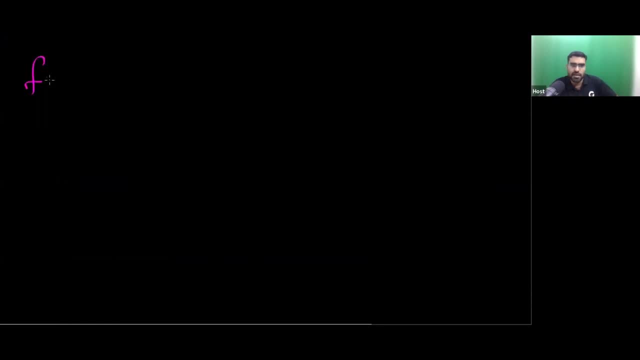 So what will be f 10?? If you notice, if you notice what is f n, that is basically f n minus one plus n minus one. or I can say what is f n plus one. Okay, So forget about this. Yeah, this is actually correct. 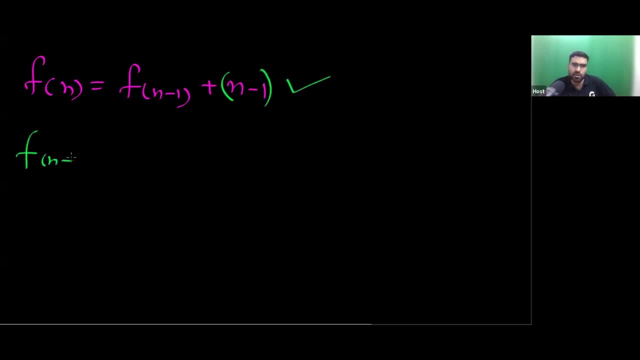 It's not wrong, This is also correct. But let's see What is f n plus one. Let's see what is f? n plus one. That is basically f? n plus n. Now, can you open it? Can you open it? 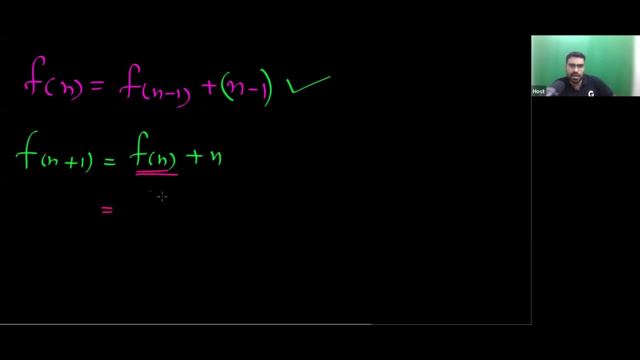 Can you open this f? n? f? n is nothing but n f n minus one f previous, plus n minus one, and this n is already there and this n is already there. Okay, Can you open this also? Can you open this also? It will be f of previous. 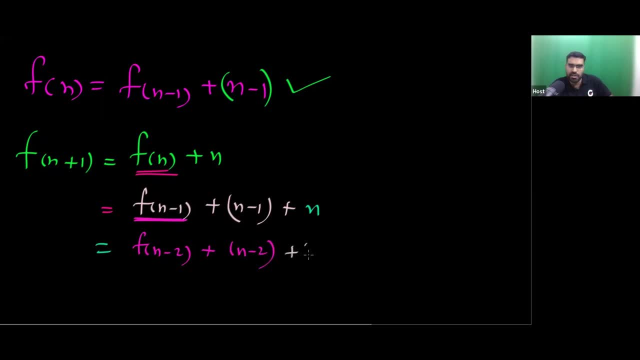 It will be f of previous, plus n minus two. This is already there. n minus one, And this is already there. If you do like this, can you see something? Can you see what is happening? n plus n plus one, plus n plus two. 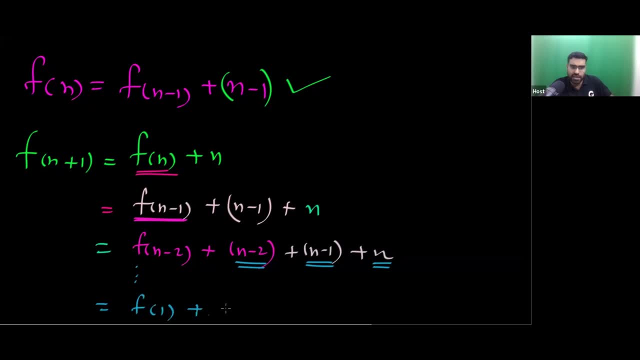 If you do like this, ultimately, if you get f one, if I get f one, then it will be like one plus two, plus and so on, n. So if you notice f n plus one, ultimately f n plus one, this and this, this is already zero. if you continue like this, if you continue like this, then this will 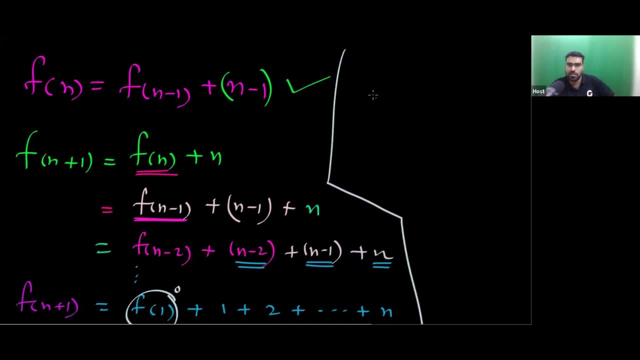 be zero. so, ultimately, what is f1 plus 1? tell me what is f? n plus 1? that is the summation from 1 to n, and this is your favorite formula, the favorite formula: n? n plus 1 by 2. this is your favorite formula and you can. now you can easily calculate anything. 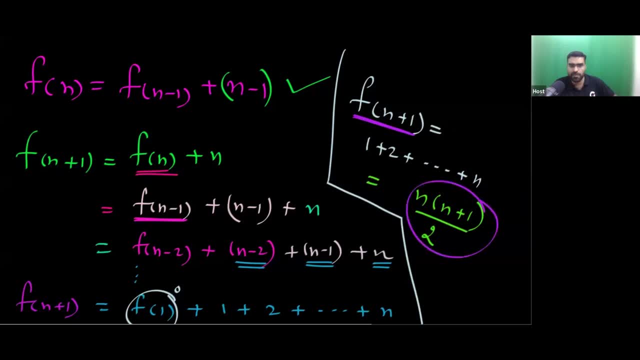 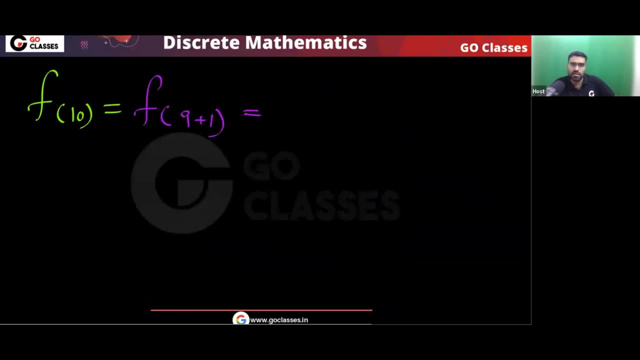 so remember: f? n plus 1, that will be n? n plus 1 by 2 f? n. so tell me what will be f 10. f 10 means f 9 plus 1, so f? n plus 1, f? n plus 1, that will be n? n plus 1 by 2. 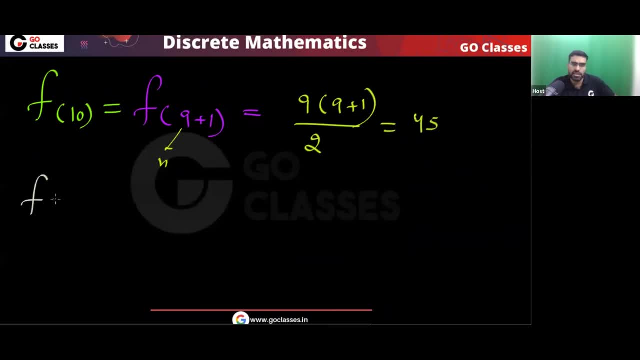 so that will be 45. you can check it out. 4, f, f, 4, f. 4 means f, 3 plus 1, so that will be 3 into 4, divided by 2, two, So that will be six. You can check it out. So this is the complete analysis of this.